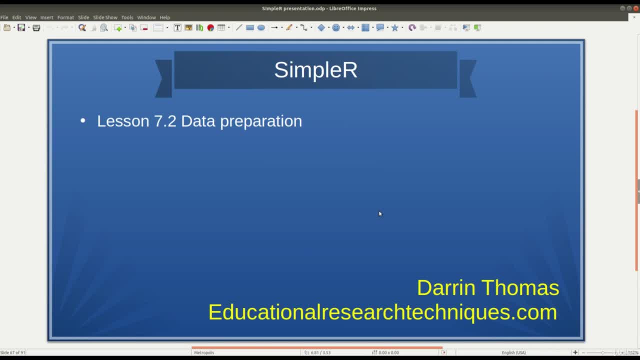 Hello, my name is Darren Thomas and I am the Director of Educational Research Techniques. This is Simpler Using Machine Learning Algorithms in R, And so now we're going to go ahead and do our data preparation. here I'm going to try to give you an idea of what our goal and our purpose is. 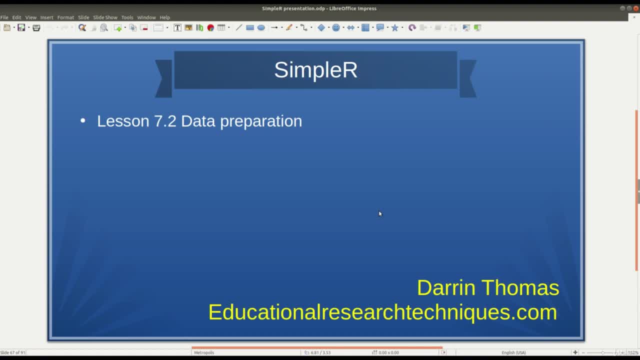 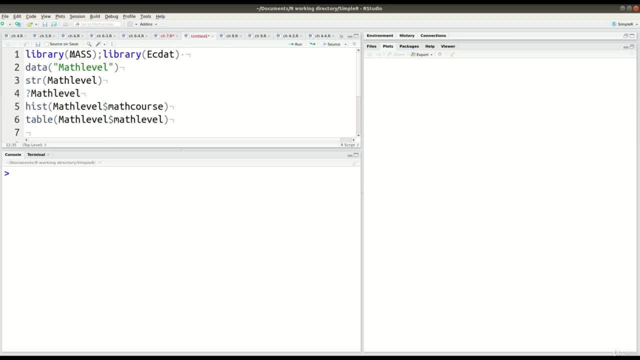 as we apply these algorithms in this particular chapter. So let's go ahead and move over to R. So I'm in R and what we're going to do here is we're going to use something called the math level data set. It's from the ECDAC library. Basically, we're going to try to predict. 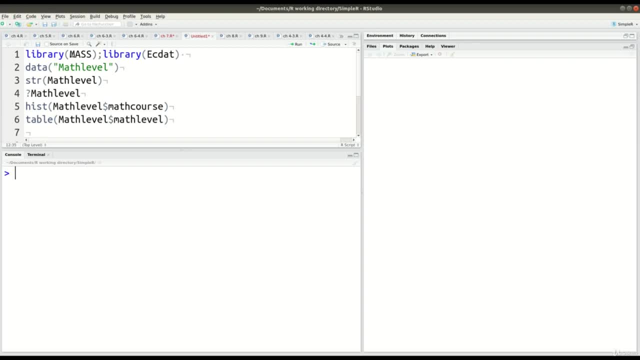 somebody's gender based on the type of classes they took and also some scores and some tests that they took as a university student. So in line one we just have the two libraries that we're going to need Packages. I guess you can call them as well. The math library has our QDA. 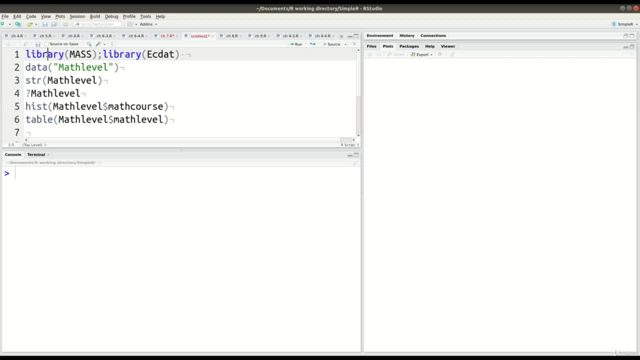 function in it and also our LDA function for quadratic and linear discriminant analysis, And the ECDAC package or library has our data set, So we'll run that nothing happens. We'll load our data set. math level- that's the name of it. 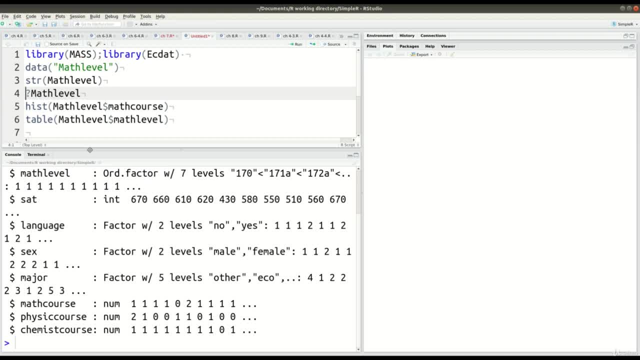 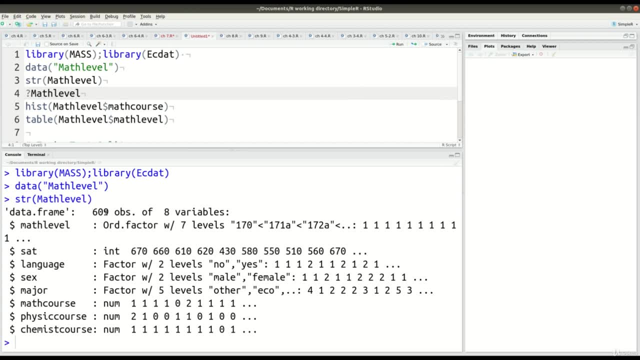 And we'll use the STR function to kind of get an idea of what's going on inside it, because I can make this a little bit bigger for you for now. Okay, so you can see, we have about over 600 samples, if you will, over eight variables. 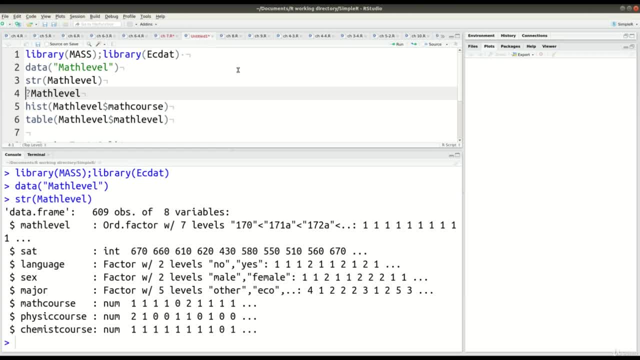 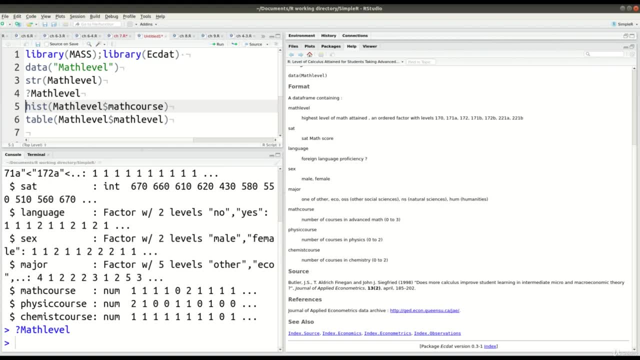 We're going to use all the variables in this particular one, And so to give you an insight into what the variables are about, we use the question mark and we type in math level, And so let me zoom this in for you so you can get a little bit of a better picture. Okay, 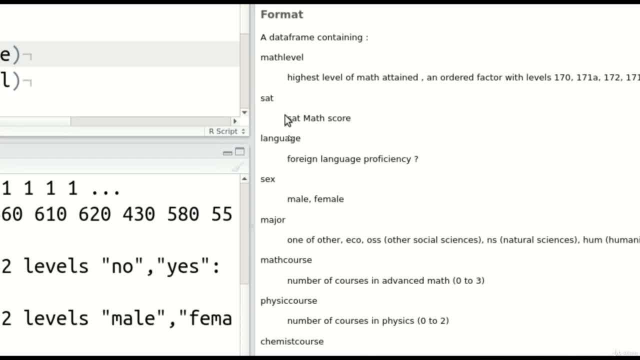 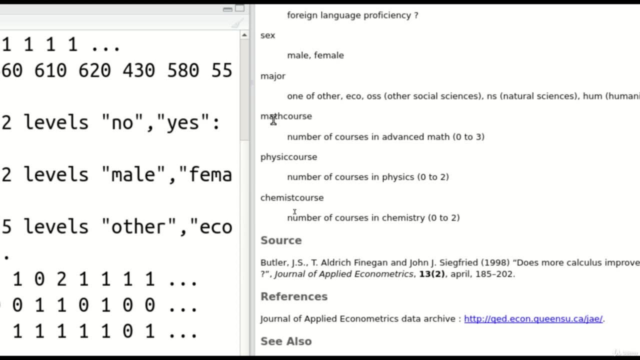 so you can see here our variables. So SAT is their math score on the SAT Language proficiency. I believe that's probably a categorical variable. Sex major math courses they're taking how many? zero to three physics courses, chemistry courses? Of course these are all classes that require a 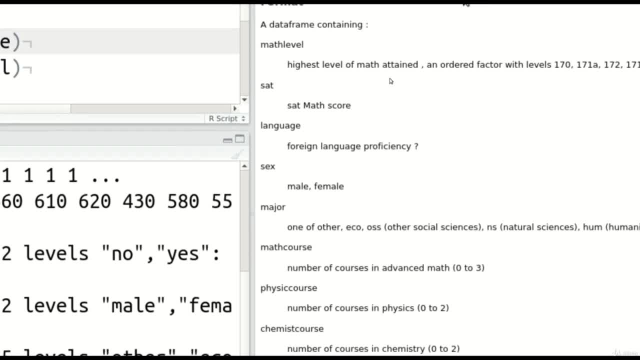 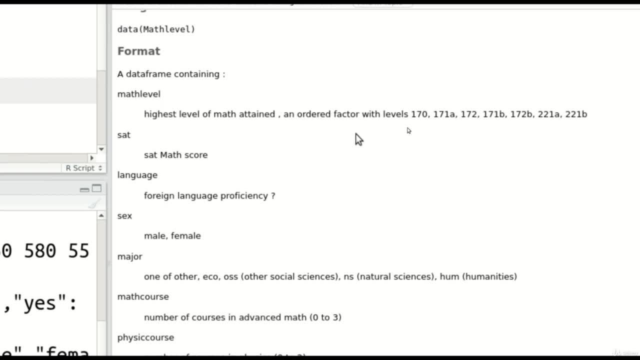 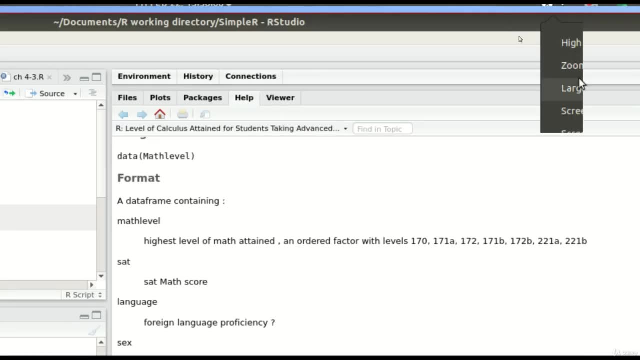 lot of math, obviously physics and chemistry et cetera. So that's kind of describing our variables in the set. We also have an ordered factor variable, math level. So obviously 170,, 171A, 172, as you go up their courses are harder probably. So that's kind of what's. 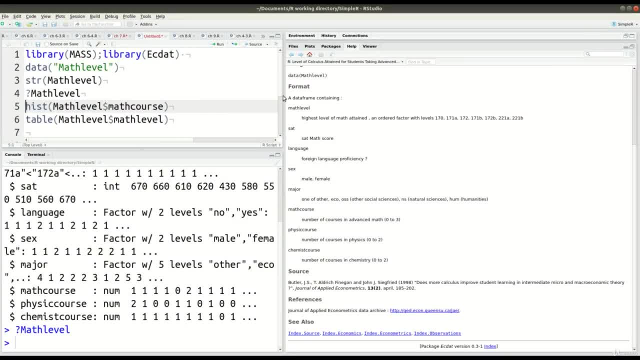 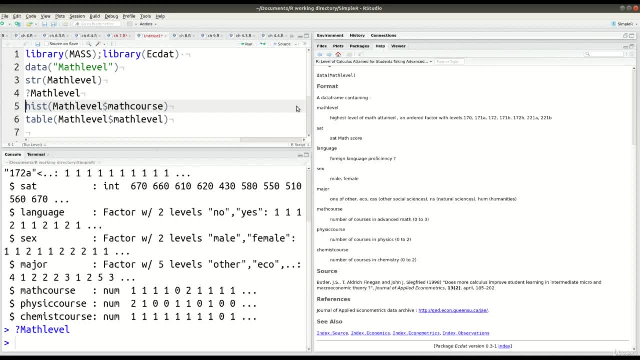 happening there. So I can make this a little bit smaller now and focus on the other side of the data. All right, oops, no, I need to deal with the histograms first. Okay, so I just want to make one or two histograms to give you an idea of the characteristics of the data, So you can see here. 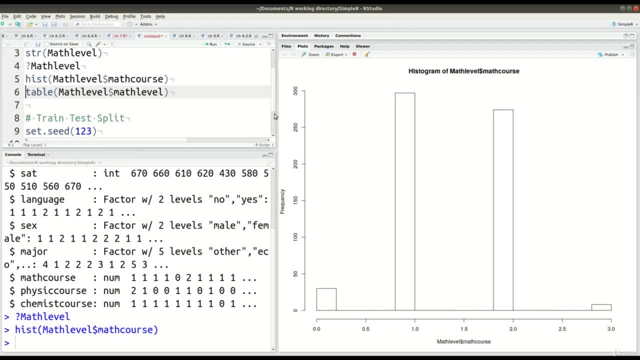 the math courses. this is almost like a factor variable, if you almost like that. So a handful of people have not taken any math courses. Most have taken one and two and then a handful have taken three. That's kind of what's happening If you look at the table for math level. 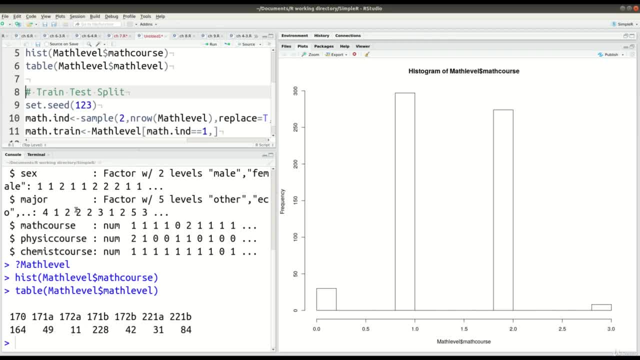 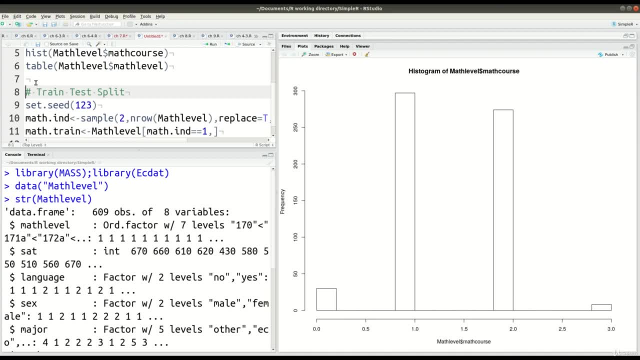 you can see here how many people were taking each class, et cetera. So that's kind of what's happening there. Again, there's not a lot of numerical stuff here. I believe maybe the SAT score. we could do that real quick. So here's. 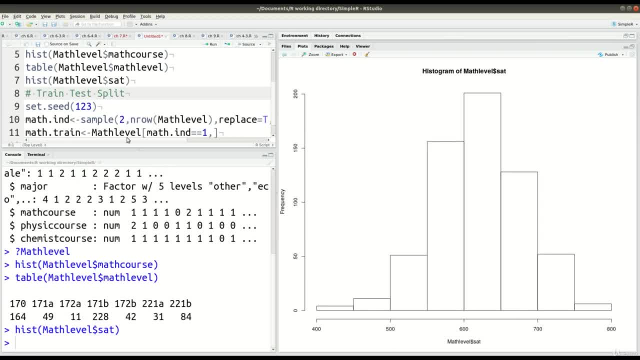 the math level SAT. we could do that, And so these are the SAT scores. Nice, beautiful little bell curve there, But again not a whole lot of exciting stuff happening here, And so with lines eight, nine, 10,, 11 through 12, we're just going to set up our train test split, and then we will. 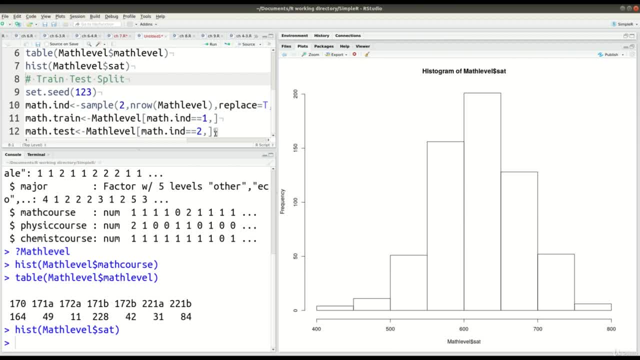 be using this data as we make our algorithm. But again, I just want to clarify something that I mentioned in the prior video, but it's so important I want to say it again: You only want to use your test set one time. This is kind of a common 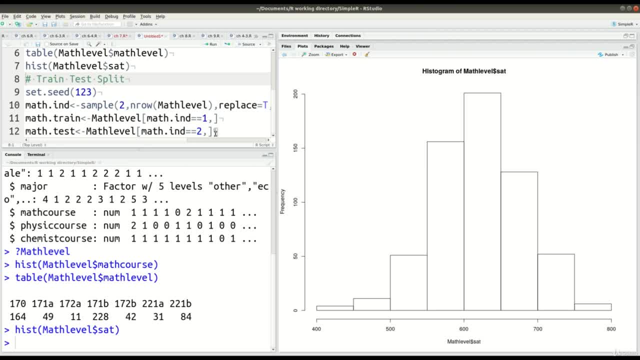 tenant of data science, machine learning, And so again, I want you to think. you have to kind of assume- because, remember, we're just practicing here- that we don't really have a test set here. we have a validation set. Often what is done is that the data is broken into three parts. 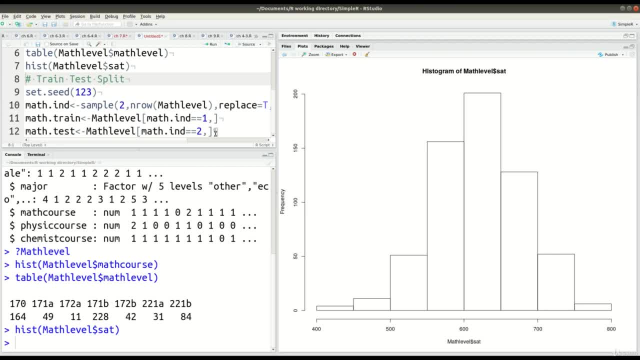 You have your training set, where you train your data. You have your validation set, kind of like a test set, if you will. And then, finally, you have your testing set. You use your validation set to try to figure out which is the best model to use on the test set. That's kind of what's happening. 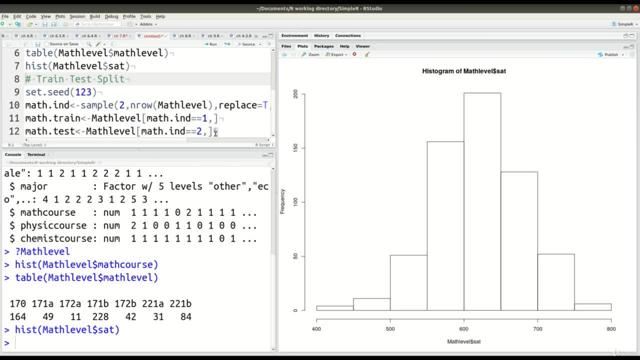 here. So again, sometimes the verbiage is not quite as accurate as we would like, but I just want to make sure that's clear, because I don't want to send people out of here with bad habits. So, having said that, the code in lines nine, 10,, 11, and 12,. we've already seen this several times. 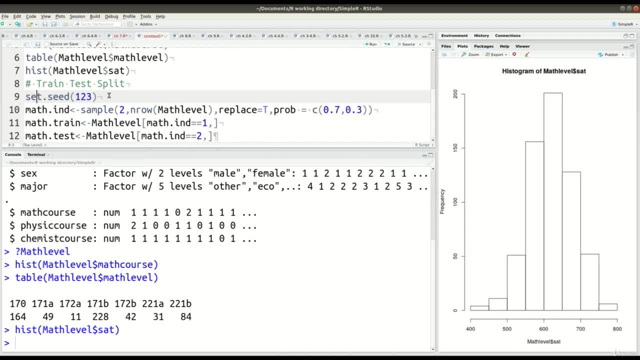 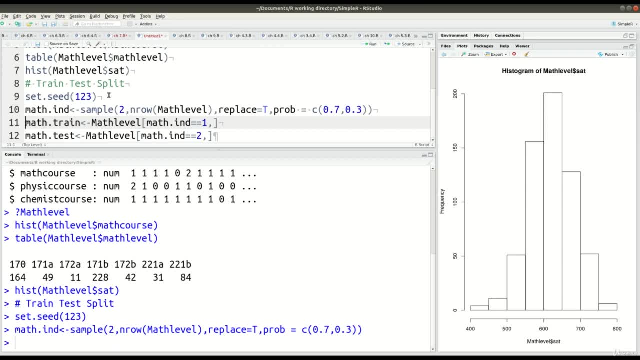 We're just rerunning it, using the stuff for this content. So we set the seed, we set up our index from one to two, one to two, How many one and twos For the same number of rows as there are in math level, and 70% of it should be ones. 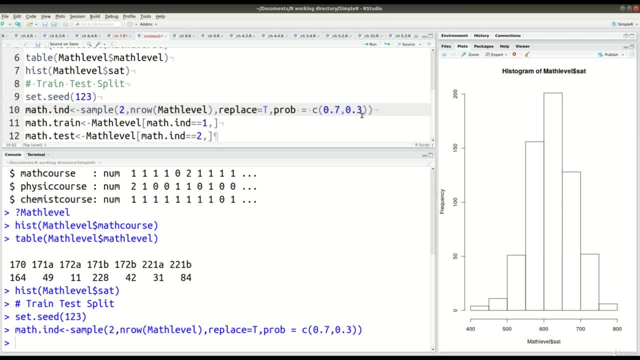 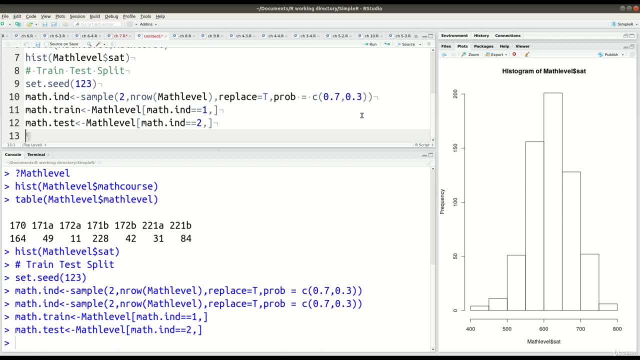 30% should be twos, because we want 70% of our data to be for training and 30% to be for validation, if you will. And so we run that, and then we set up our data sets, mathtrain, mathtest, and we're ready to go. So in this video, all we did was- you know, 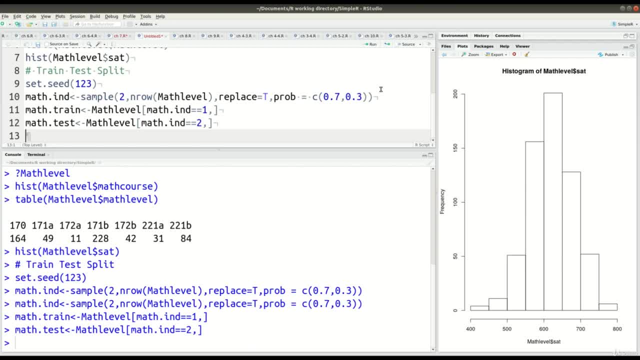 I exposed you to the data set that we're going to be using math level. We're going to be trying to predict gender based on the type of math classes they took, their math SAT score, their language proficiency, et cetera. I explained to you, or we looked at, some of 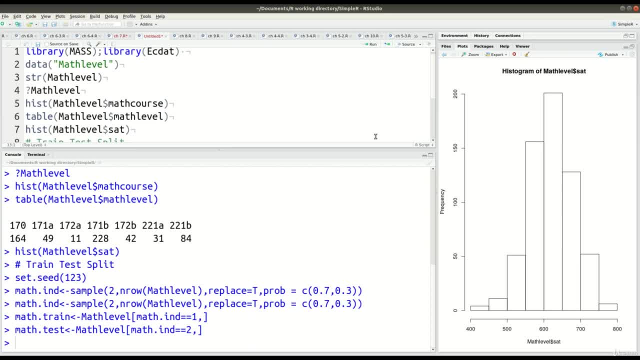 the visualizations for some of the variables, and I also tried to clarify the importance of understanding that what we're really doing here is a training. then we move to a validation. We're not really doing testing, because when you're using multiple models, remember you only. 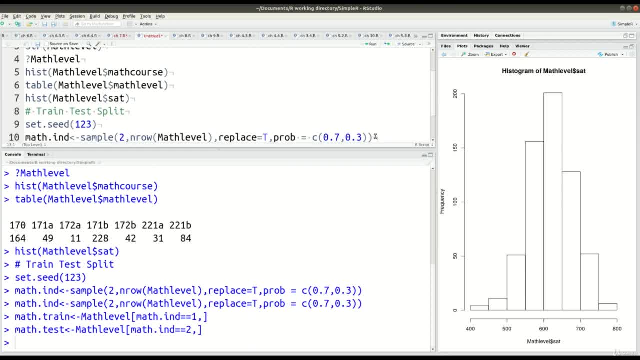 only want to use your test data one time. Otherwise, you begin to train your data on the testing data, which is not you're not supposed to do that. So I hope this video was useful for you in that you were able to understand what we were talking about here. 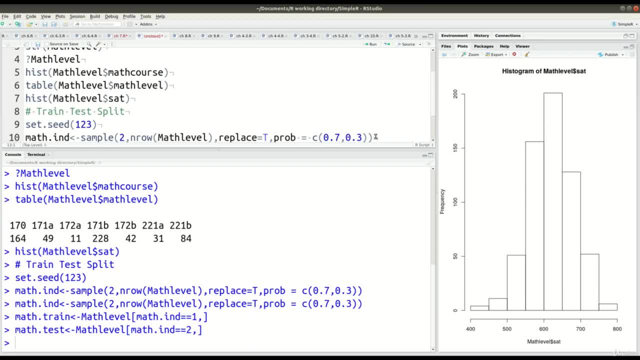 So my name is Darren Thomas. I am the Director of Educational Research Techniques. This is Simpler Using Machine Learning Algorithms in R. Take care.